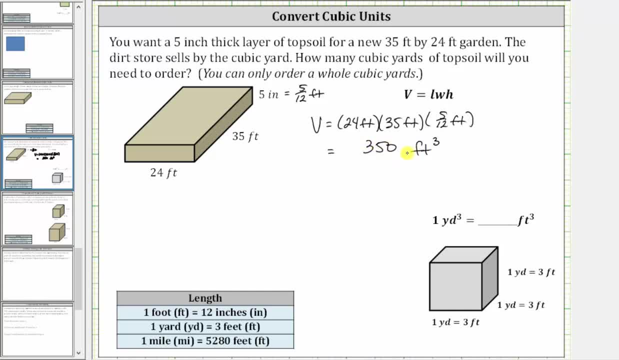 And now let's convert the cubic feet to cubic yards. but before we do this, let's determine the conversion from cubic yards to cubic feet. Looking at this cube, notice how the dimensions are: one yard by one yard by one yard, This is one cubic yard. 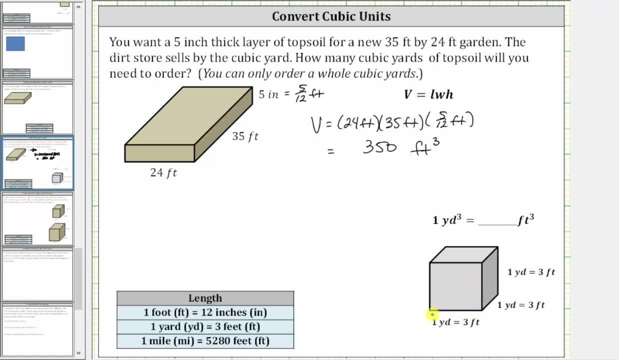 And since one yard is equal to three feet, we can also label the dimensions three feet by three feet by three feet, And therefore in cubic feet. the volume is three feet times three feet times three feet, which gives us 27 cubic feet. 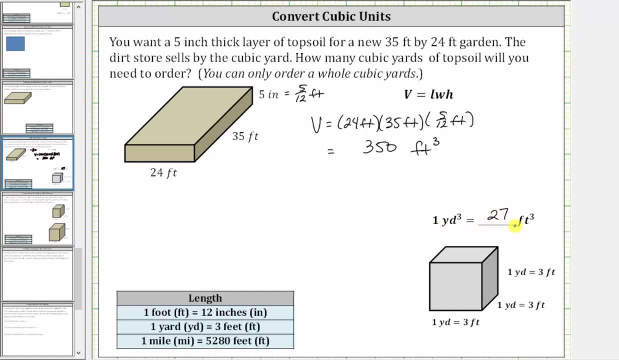 So now we know one cubic yard equals three feet. times three feet, That's equal to 27 cubic feet. Let's use this to convert 350 cubic feet to cubic yards. Let's first write 350 cubic feet as a fraction, with the denominator of one. 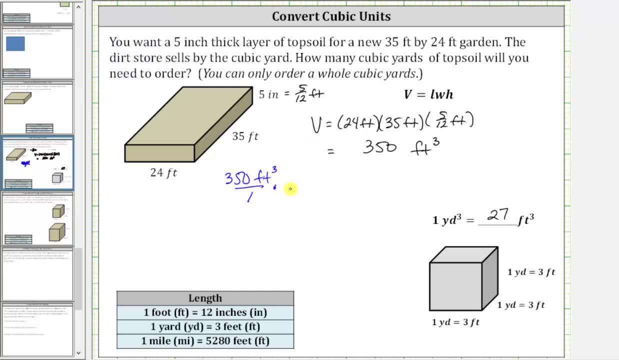 And now we will multiply by unit fraction to convert cubic feet to cubic yards To form the unit fraction. because we have feet in the numerator and we want cubic feet to simplify out, we must have cubic feet in the denominator of the unit fraction. 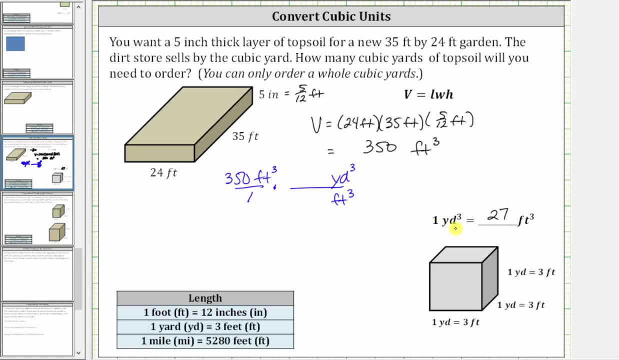 and cubic yards in the numerator And since one cubic yard is equal to 27 cubic feet, the unit fraction is one cubic yard over 27 cubic feet, Because we have cubic feet divided by cubic feet. the units of cubic feet simplify out. 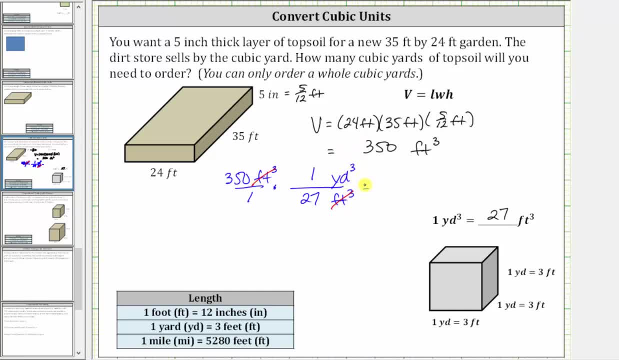 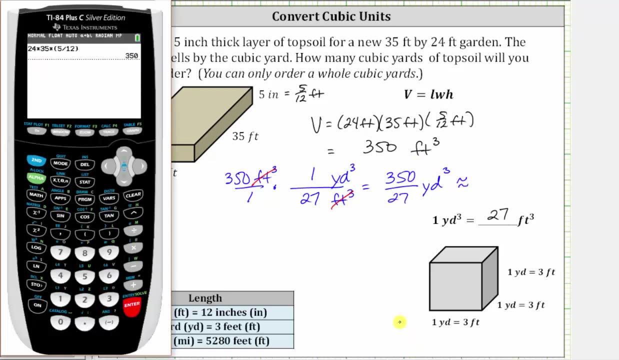 leaving us with cubic yards. So now multiplying. notice how we have 350 over 27 cubic yards. Let's go back to the calculator and determine this quotient: 350 divided by 27 is approximately 12.96.. Of course, it's still cubic yards. 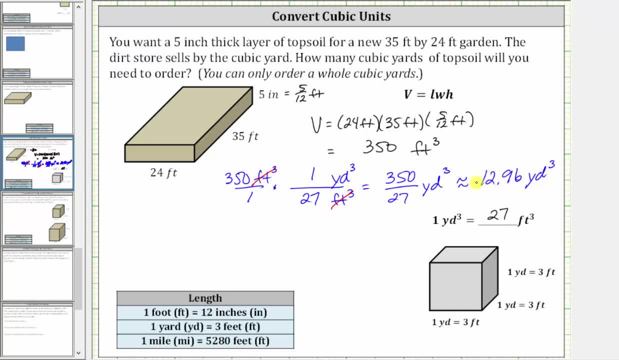 But remember, we can only order whole cubic yards and therefore anything over 12 cubic yards, we would have to order 13 cubic yards. You must order 13 cubic yards. So remember, even if this was, let's say, 12.1 cubic yards, 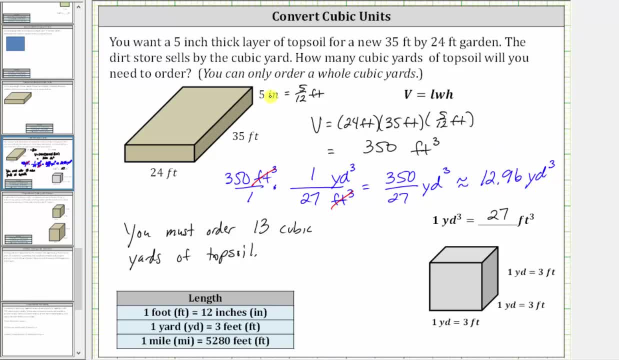 you would still have to order 13 cubic yards, because you can only order a whole number of cubic yards and if you ordered 12, you wouldn't have enough. I hope you found this helpful.